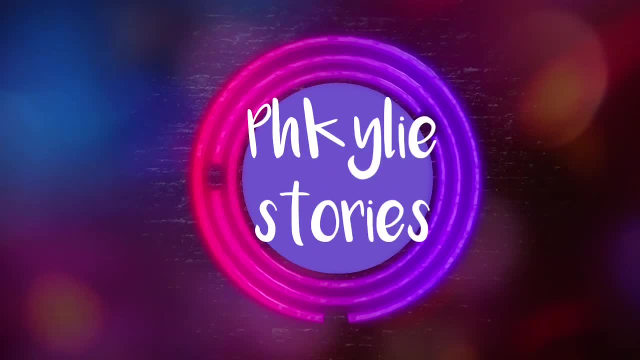 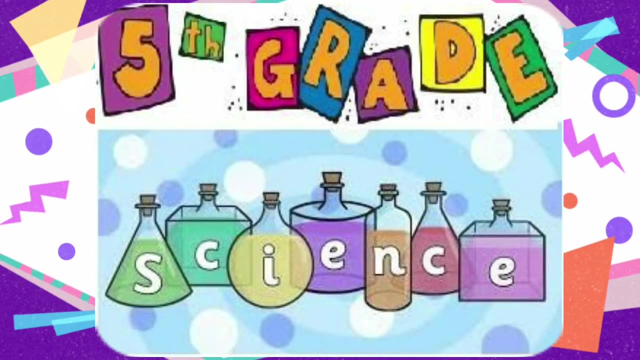 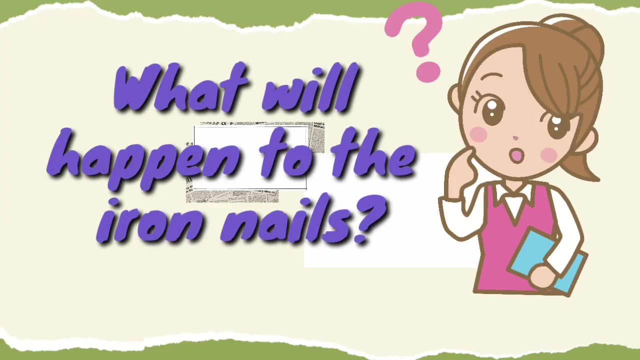 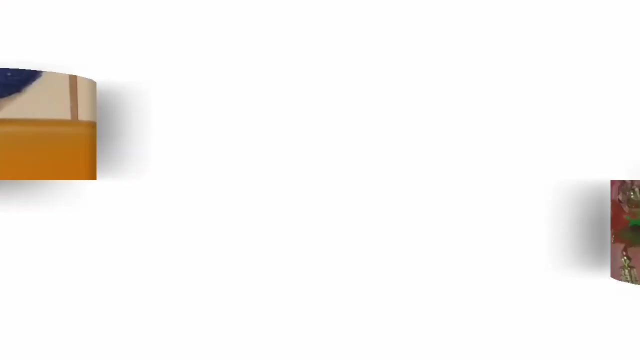 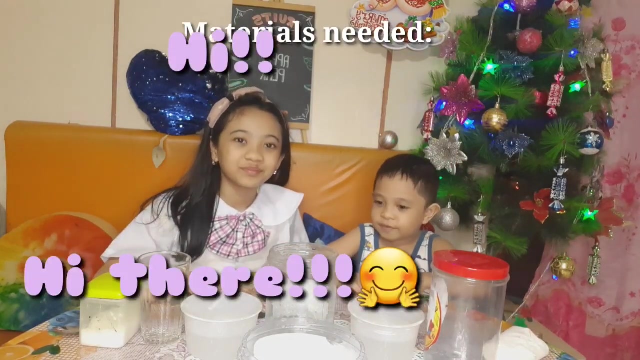 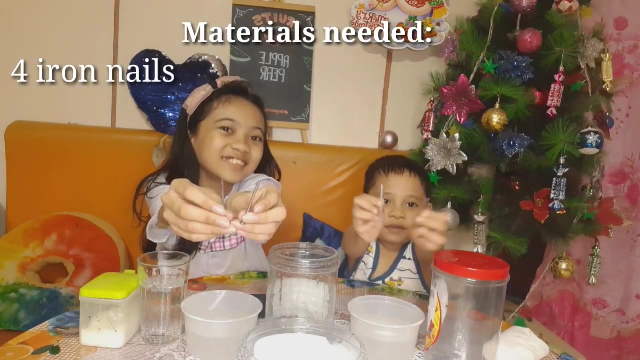 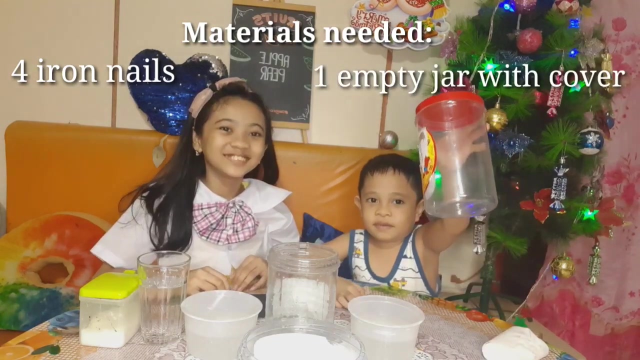 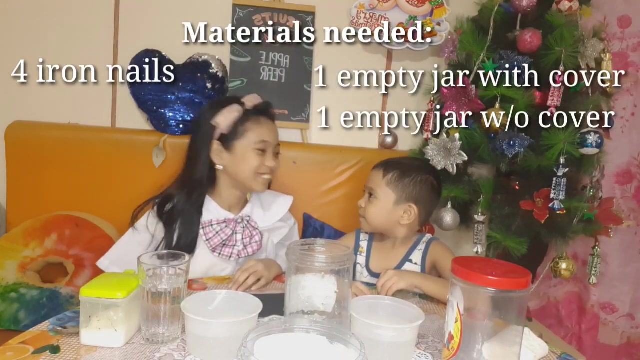 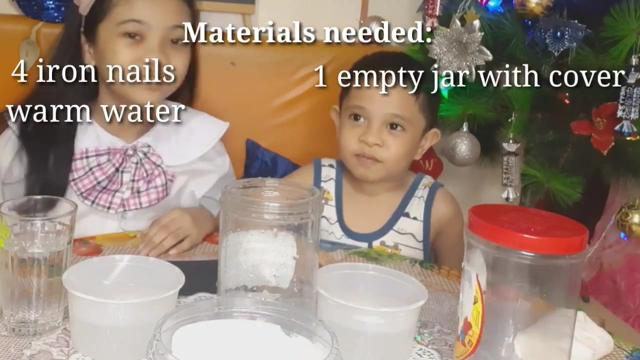 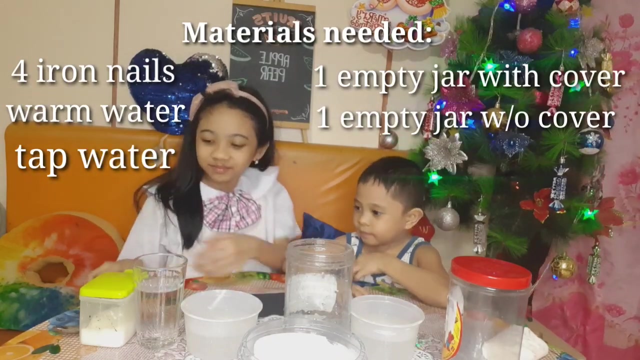 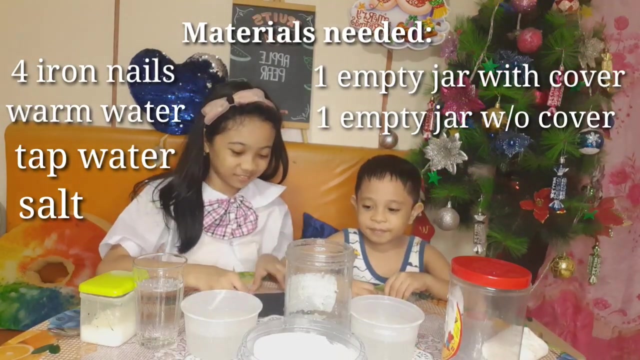 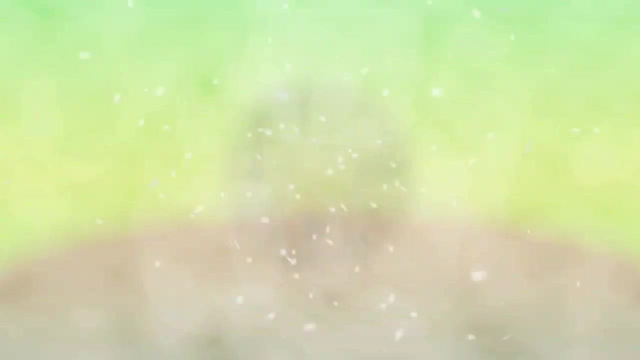 Hi, Hi there. Materials Needed: 4 Iron Nails, 1 Empty Jar with Cover, 1 Empty Jar without Cover, Warm Water- Make sure that the warm water is not too hot- Tap Water, Salt and Sandpaper. What to Do? Step 1: Remove any rust from the nails using sandpaper. 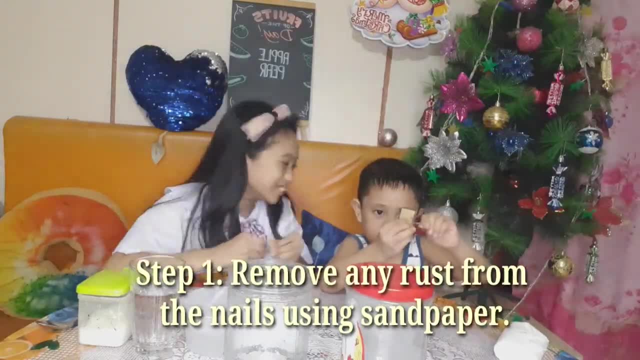 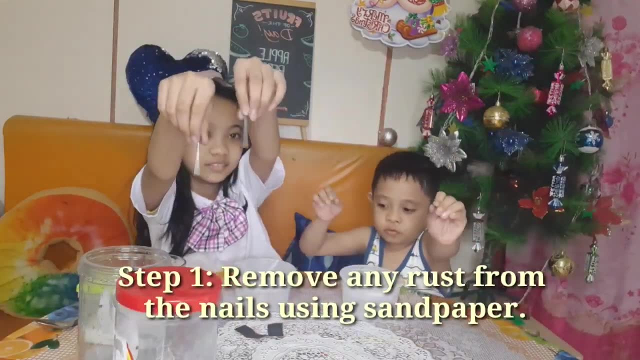 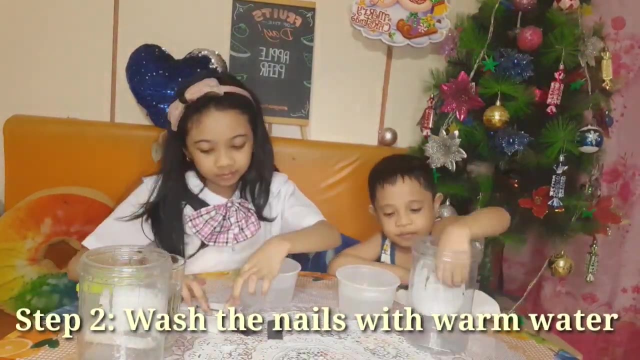 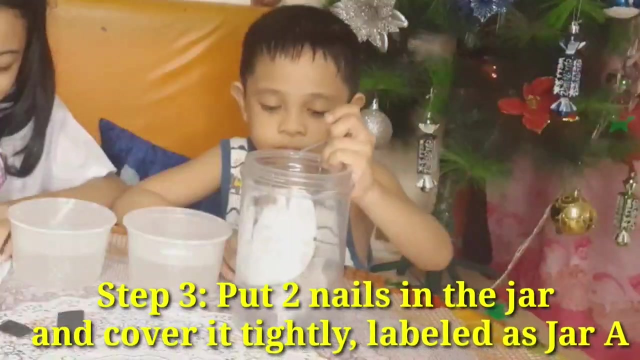 Step 2: Wash the nails with warm water. Step 3: Put two nails in the jar and cover it tight. LegalJazzJarA, LegalJazzJarA, LegalJazzJarA, LegalJazzJarA, LegalJazzJarA, LegalJazzJarA. 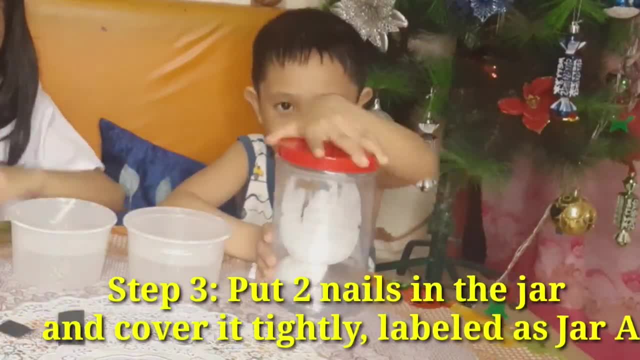 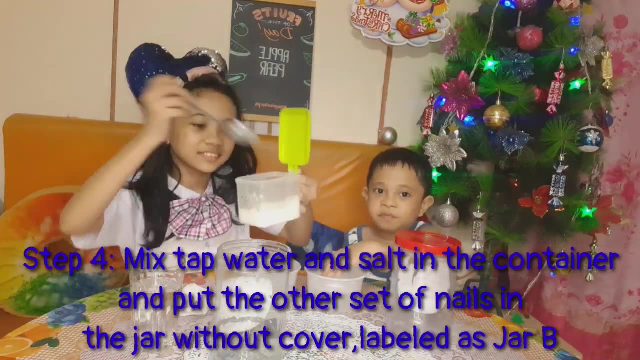 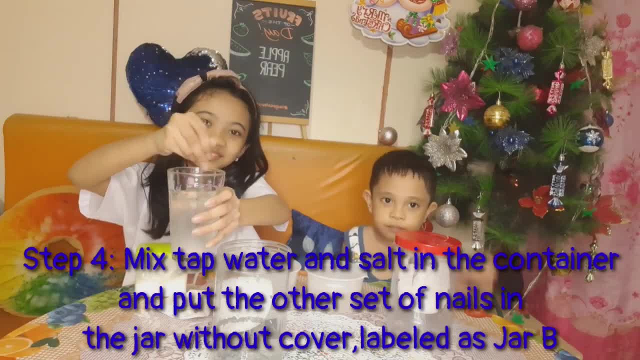 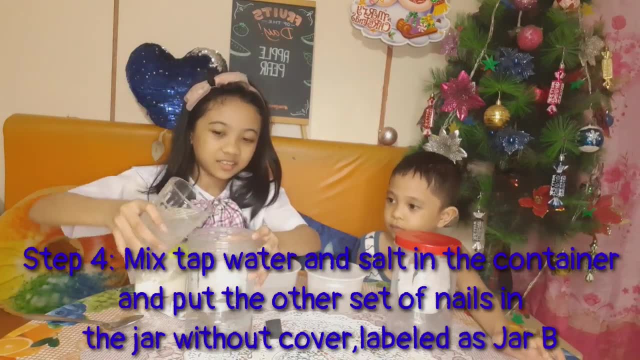 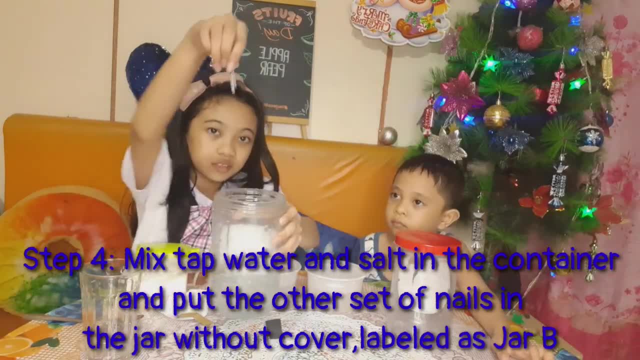 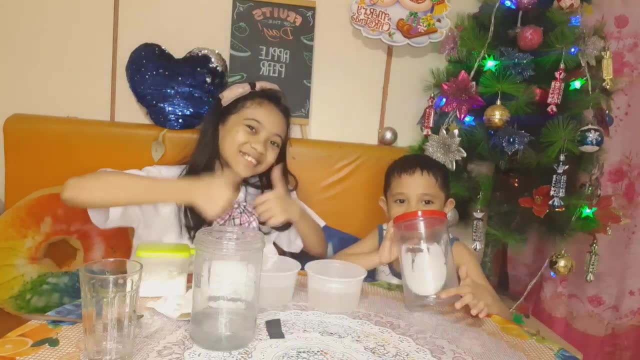 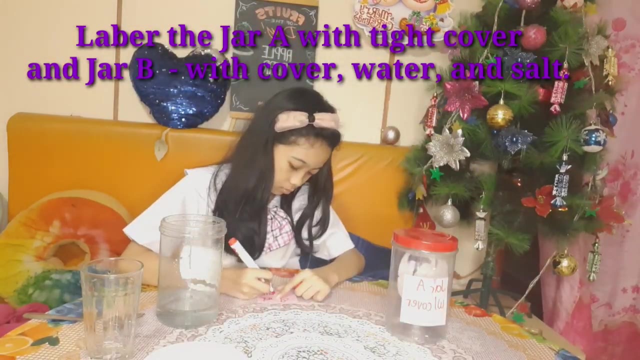 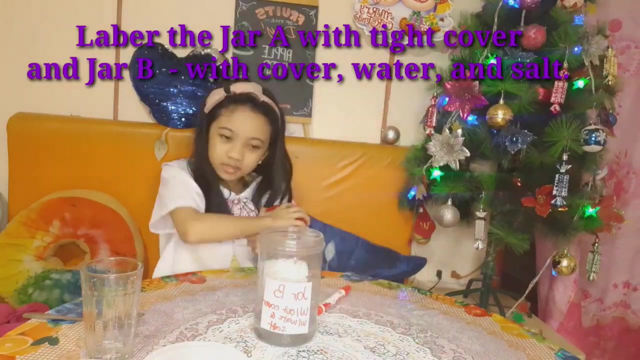 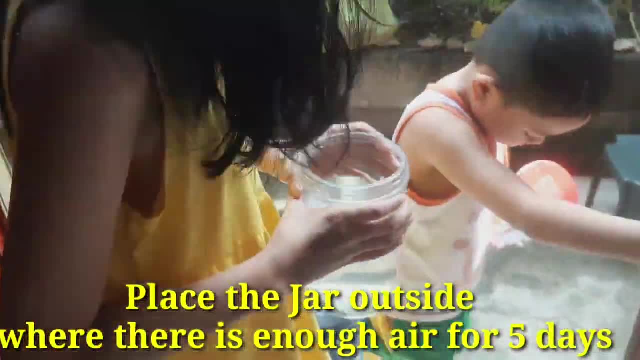 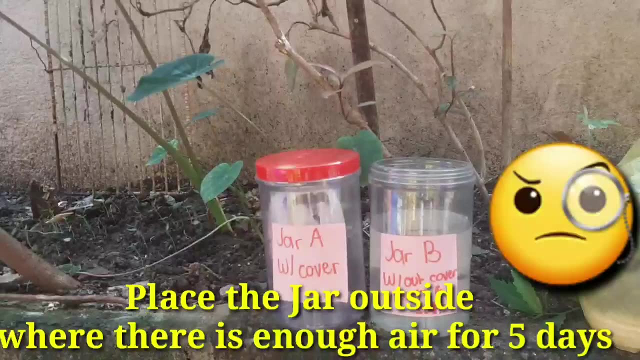 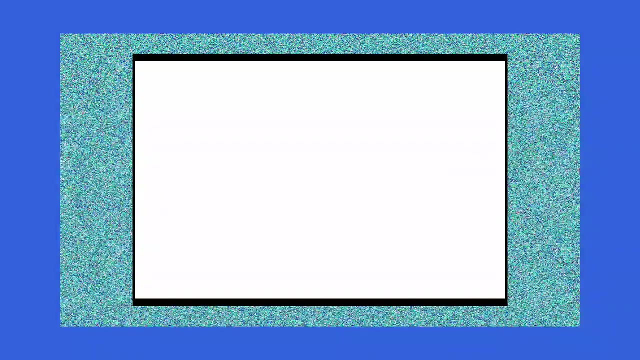 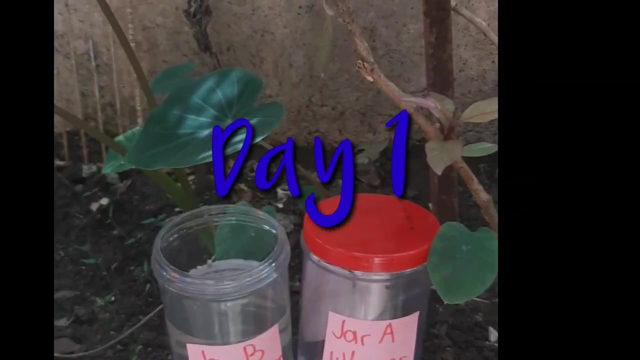 Place the jar outside where there is enough air for 5 days. Observe both jars to see what will happen to the mules. Day 1, 1st day, 2nd day, 3rd day, 4th day, 5th day. 6th day, 7th day, 8th day, 9th day, 10th day, 12th day, 11th day, 12th day, 11th day, 16th day, 18th day, 10th day, 16th day. 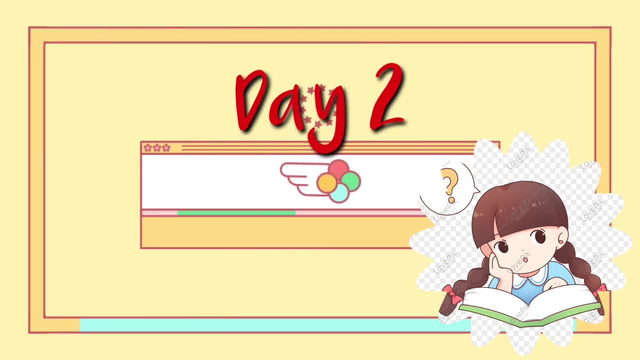 19th day, 19th day, 20th day, 23rd day, 25th day, 26th day, 21st day, 7th day. Ease up the course of about 10-30 minutes and make sure it should be still. 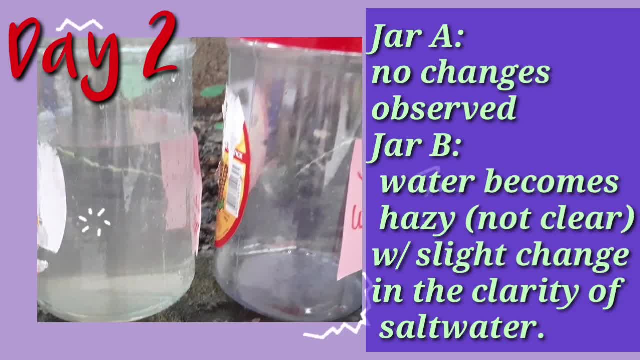 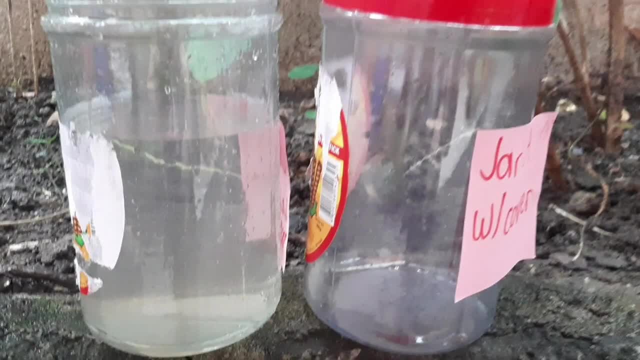 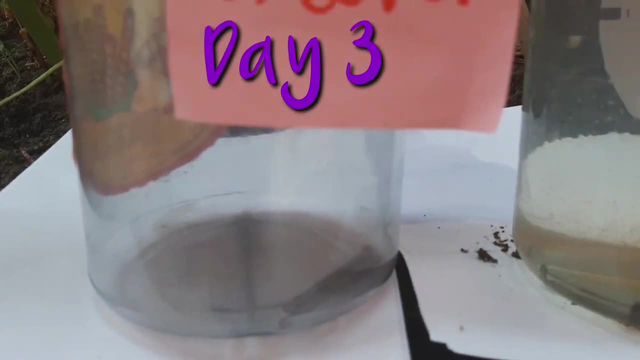 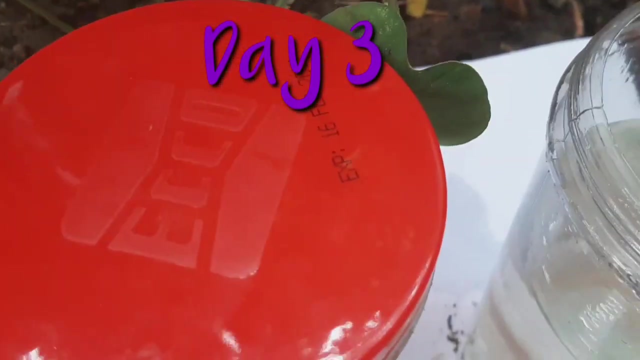 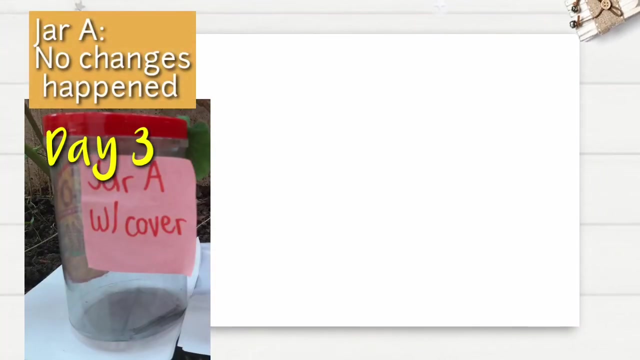 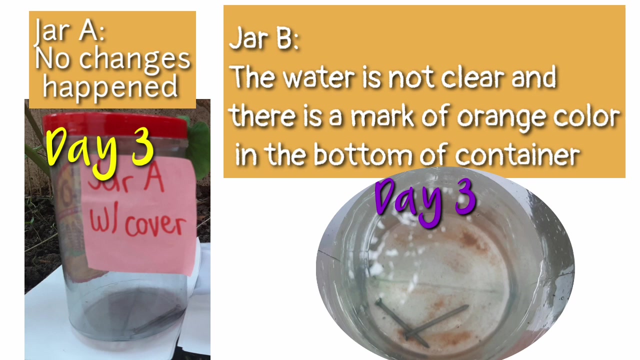 Jar A: No changes observed. Jar B: Water becomes hazy, not clear, With slight change in the clarity of salt water. Day 3: Jar A: No changes happened. Jar B: The water is not clear and there is a mark of orange color in the bottom of container. 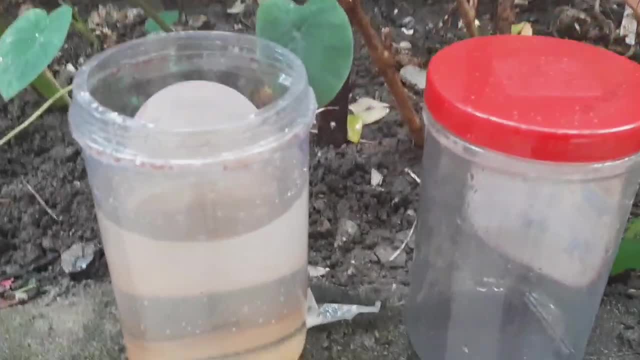 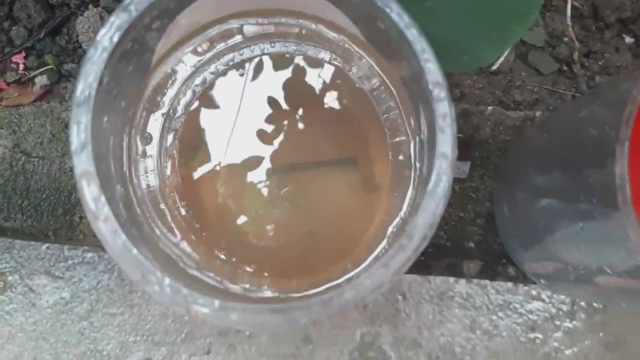 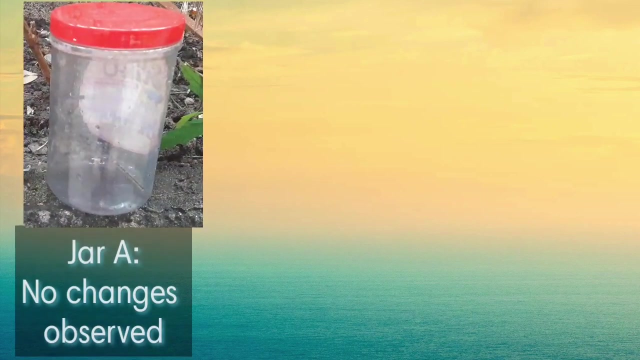 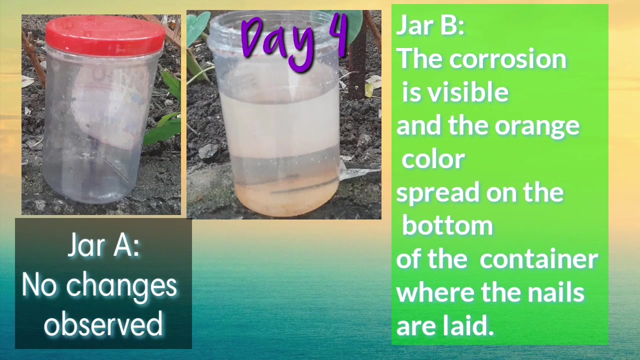 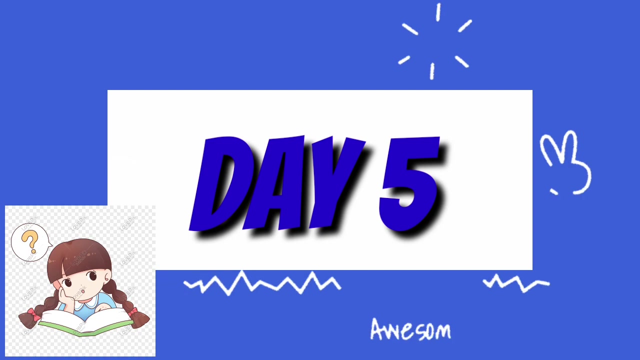 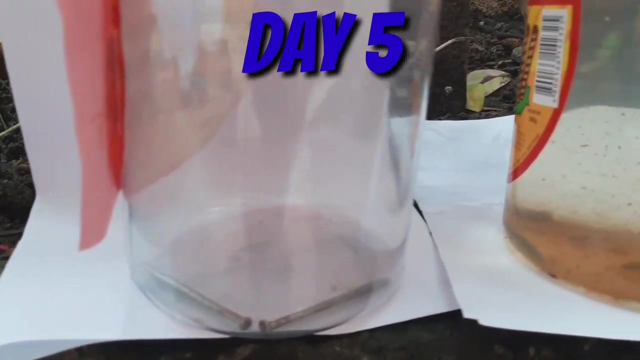 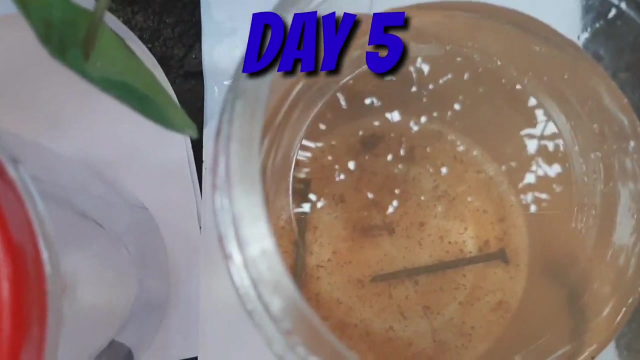 Day 4: Jar A: No changes observed. Jar A: No changes observed. Jar B: The corrosion is visible and the orange color spread on the bottom of the container where the nails are laid. Day 5, Jar A: No changes observed. 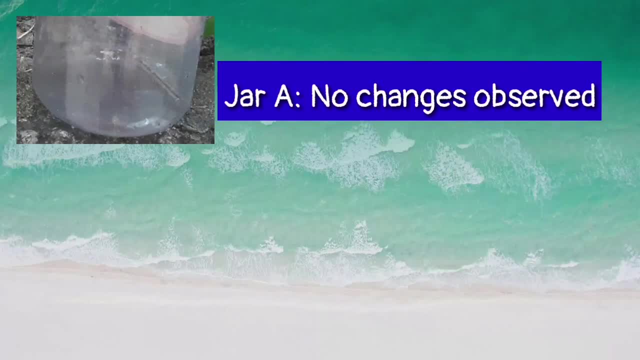 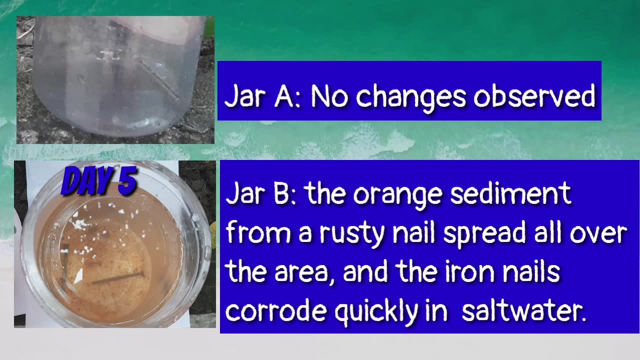 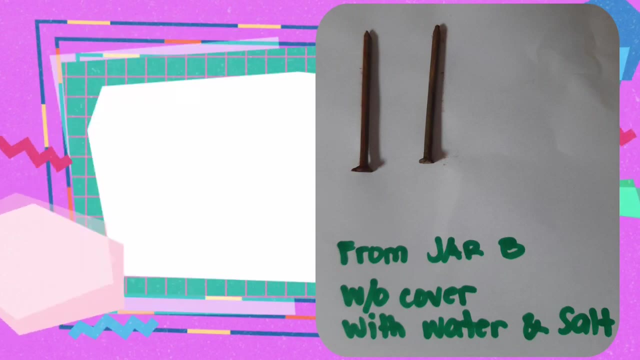 Jar A: No changes observed. Jar B: The orange sediment from a rusty nail spread all over the area and the iron nail corrode quickly in salt water. corrode quickly in salt water As a result after 5 days of experiment. jar A with cover.